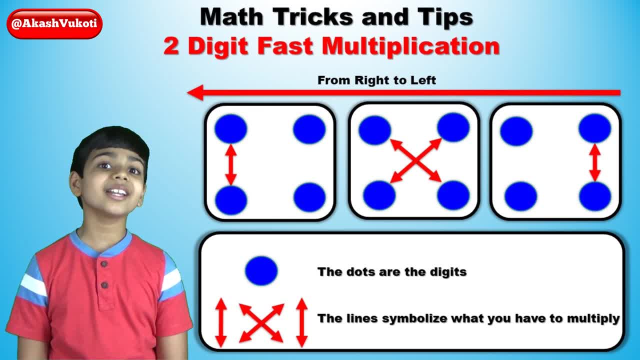 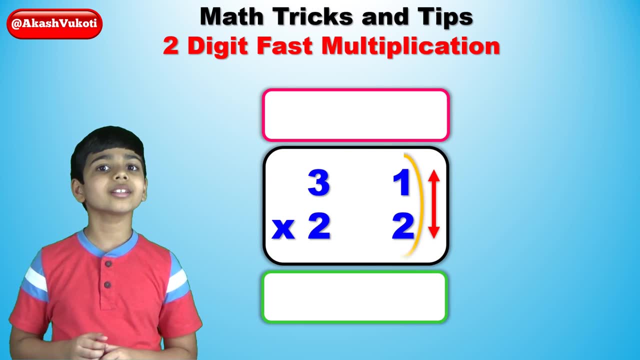 As you can see right here, the dots are the digits and the lines symbolize what you have to multiply. Write 31 times 22, like this: 31 on the top and 22 on the bottom. Let's, Let's go from right to left and multiply one times two, which is two, as shown in the 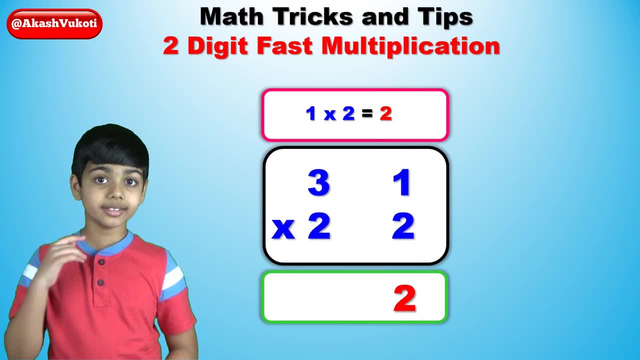 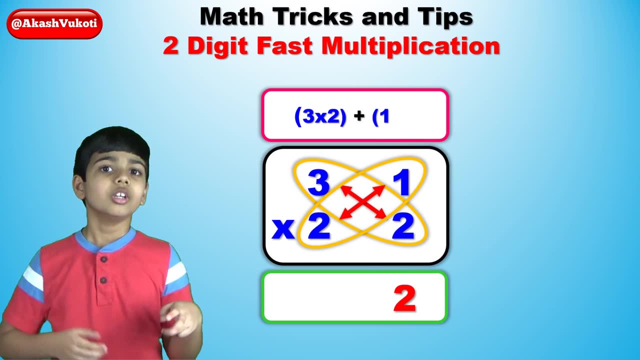 right diagram, Right two as the last digit. Now, following the middle diagram, multiply three times two and one times two, which are six and two respectively. Add these two together and you have eight. the next digit, The first digit, is found by multiplying the left most column. 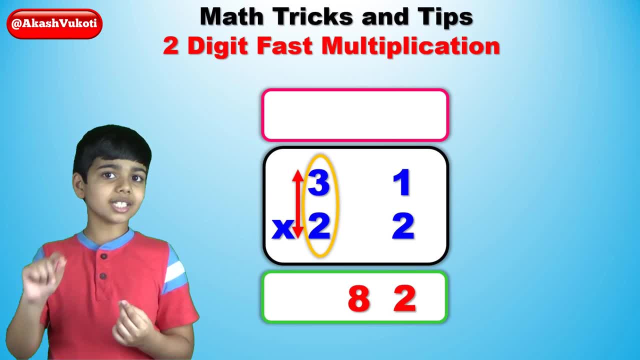 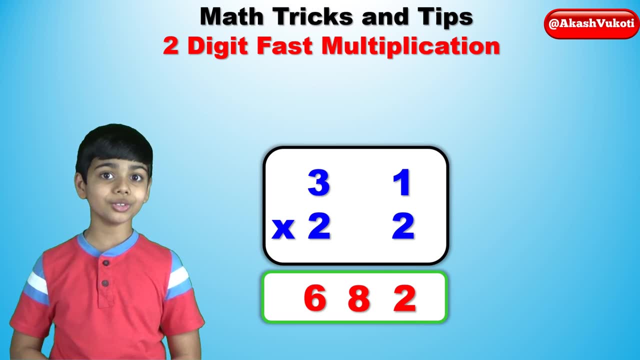 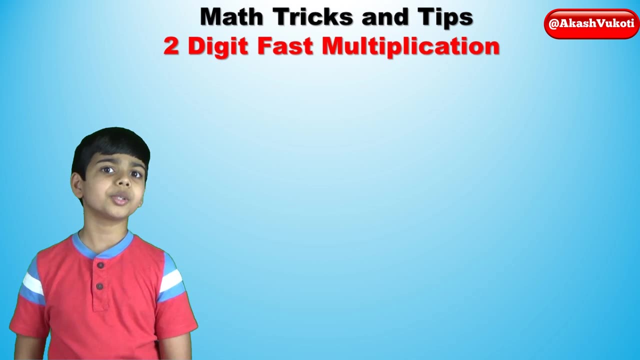 As you can see here in the diagram, that's three times two, which is six, the first digit. So thirty-one times twenty-two is six hundred eighty-two. Now let's look at the second way. Write the problem horizontally like this, instead of the first method where we put one. 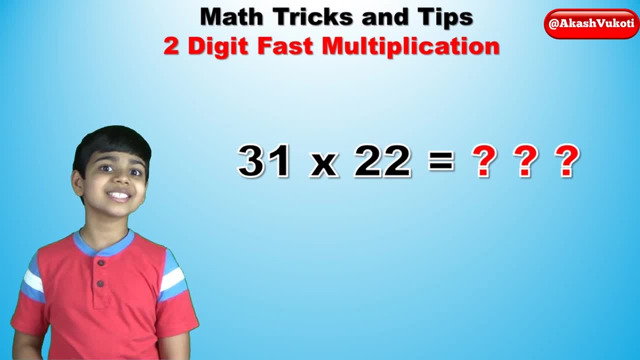 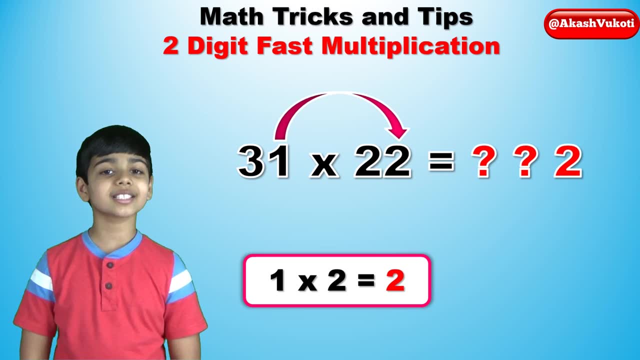 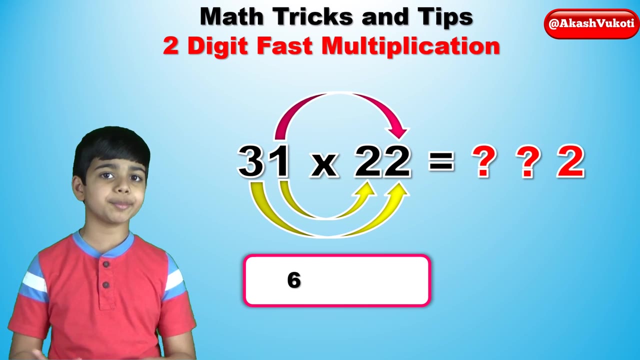 on top of the other. First, multiply the last digits of both the numbers together. So multiply one times two, which is two. That's the last digit. Next multiply three times two and one times two, which are six and two respectively. 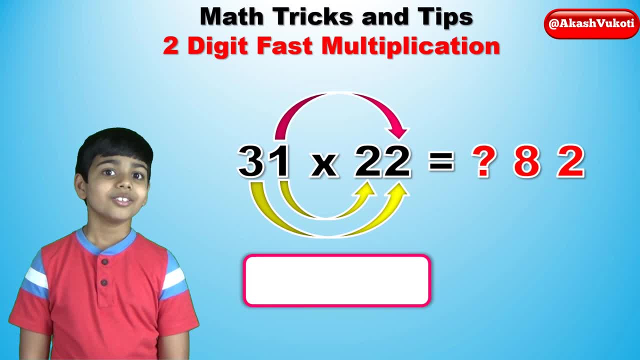 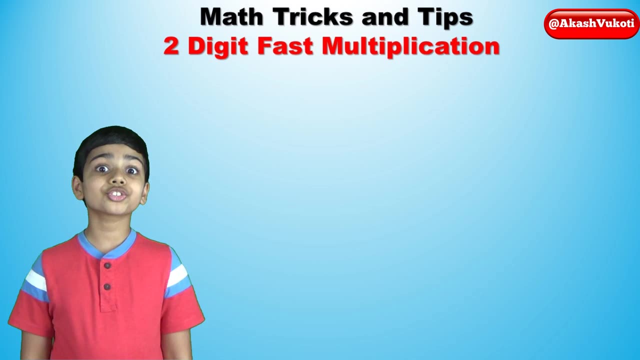 Add them together to get the middle digit eight. Finally, multiply the first digits of both numbers. So multiply three times two, which is six. That's the first digit. So the answer is six hundred eighty-two. Let's try another example. 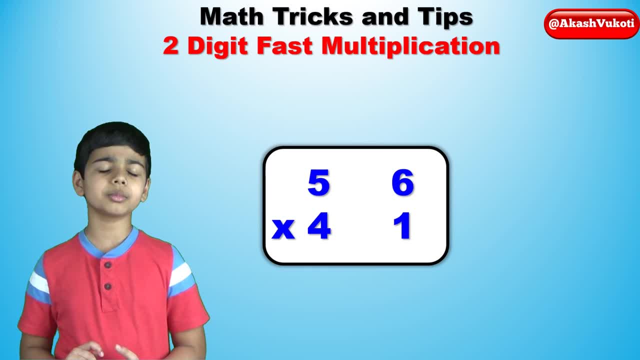 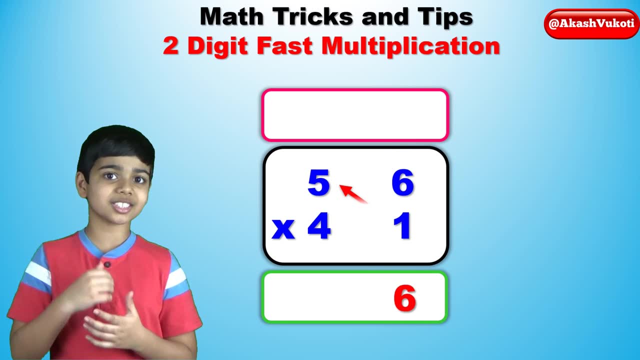 Say fifty-six times forty-one. For this problem we'll use the first method. Let's begin by multiplying six times one, which is six. Five times one is five, and six times four is twenty-four. So add five and twenty-four and now you have twenty-nine.